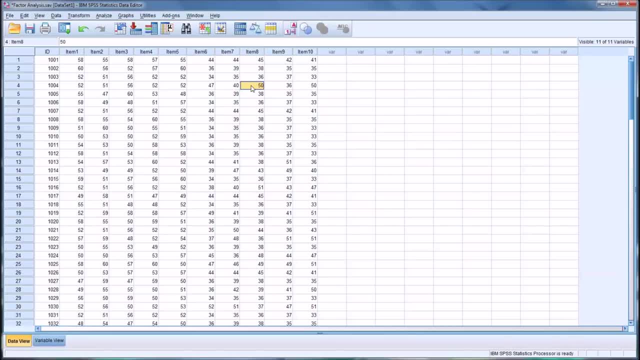 group together and or items 6 through 10 group together. That is, do those items have factor loadings which indicate that they stick together? they represent they load on the same construct. Now you could also run a factor analysis without having any idea formed in advance about how the items are going to. 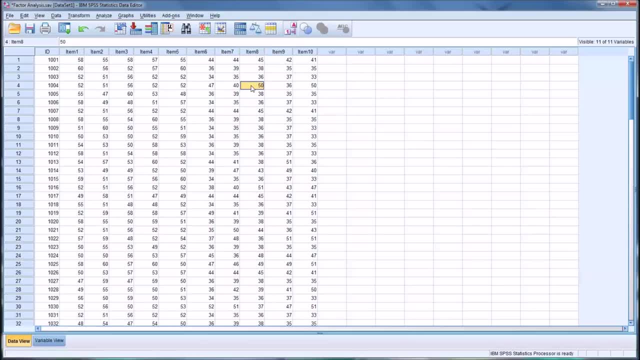 divide up. You may have some different hypotheses about how they're going to load and if they're going to load together or not, and what ways they'll load together. but you may not know. you may not have designed the instrument with a specific factor loading model in mind, So it's more. 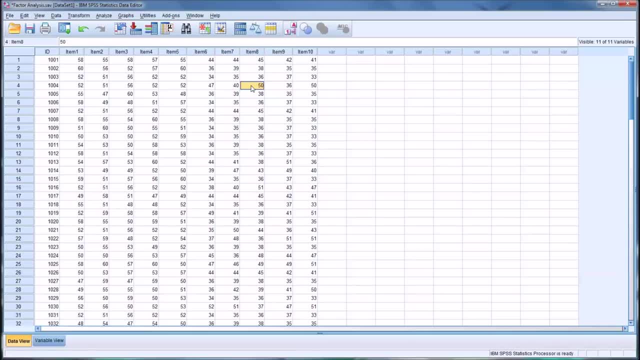 exploratory. You want to see the constructs, or if the items load together on the particular constructs. But for the purposes of this demonstration, let's assume that we designed this instrument to capture those two distinct constructs, depression and anxiety. So we would hope to see that items 1 through. 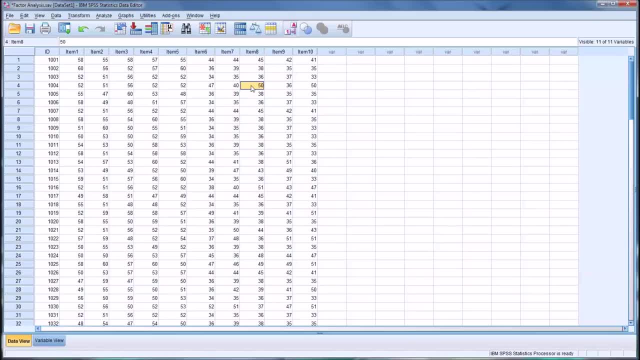 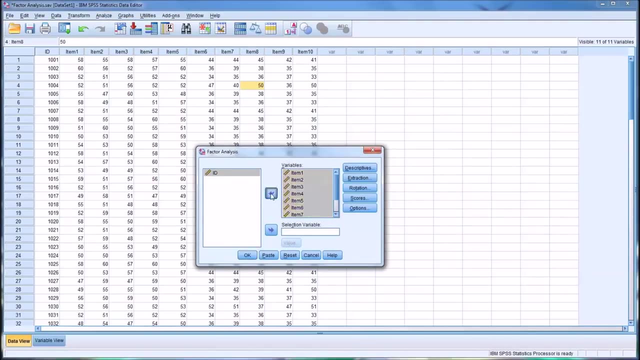 5 load together and items 6 through 10 load together. So let's start by clicking Analyze And go to Dimension, reduction and factor And you can see that. so let me put these back where they were. You can see that you have variables here. You have ID and the ten items. 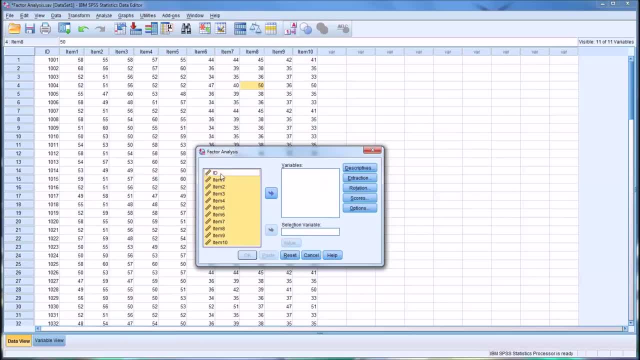 So what you should do is just select all and then deselect ID And then move them all over into the variables. So in a factor analysis, all the responses, all the individual values for the different are actually entered into this, actually loaded into this variables list box. 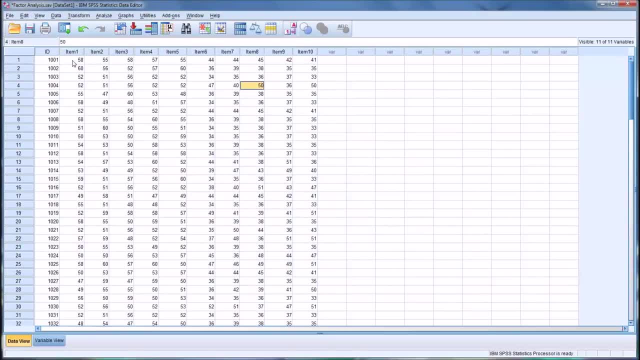 right. so to go back for a second, these, these items are actual scores, so this- this item is- might be a question related to sleep patterns, which have been tied to depression. this item might be an item that asks about not having enjoyment in in activities that once provide an enjoyment right. other criteria for 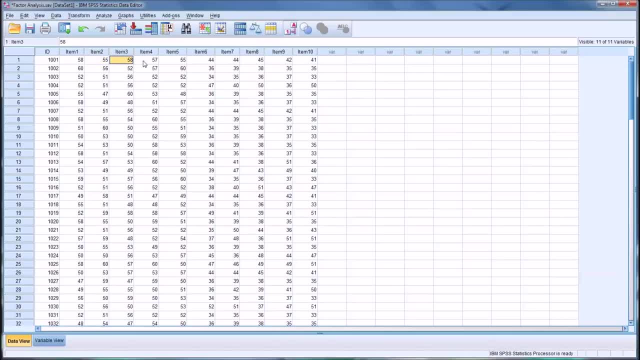 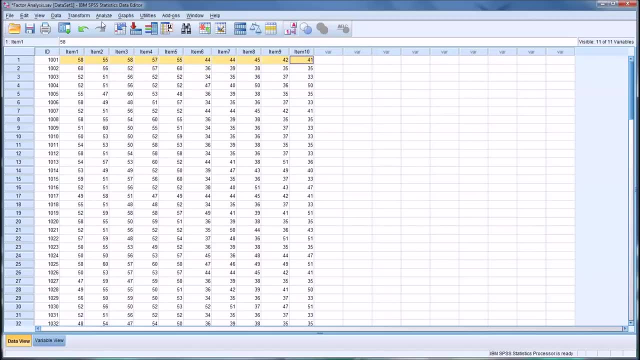 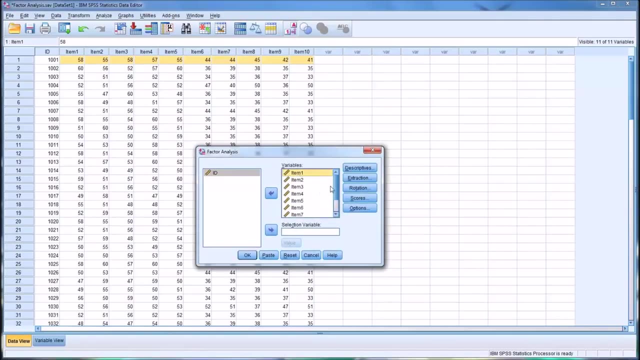 depression. so these are actual individual items or questions on an assessment, right? so you have to record them in this way in order to run a factor analysis. so, moving back to dimension, reduction and factor, so you'd have all these different items in you, the variables list box for descriptives, you're going to want the initial. 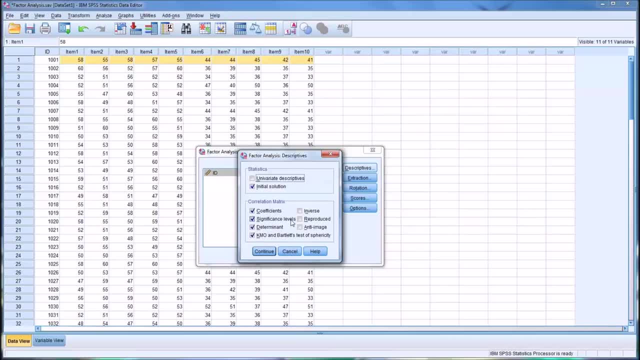 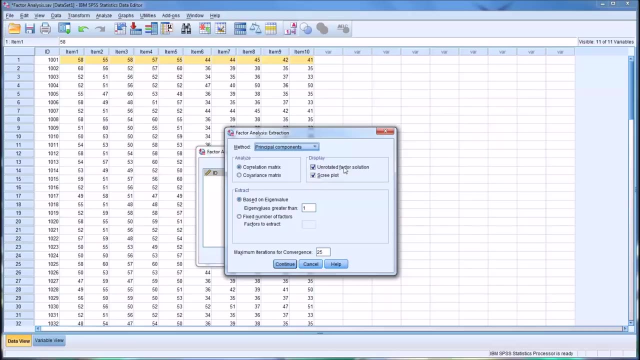 solution coefficients, significant levels to determine and camo and Bartlett's test of sphericity continue for the extraction by default, the unrotated factor solution comes up. you also want the scree plot and I left this to the default based on the eigenvector. 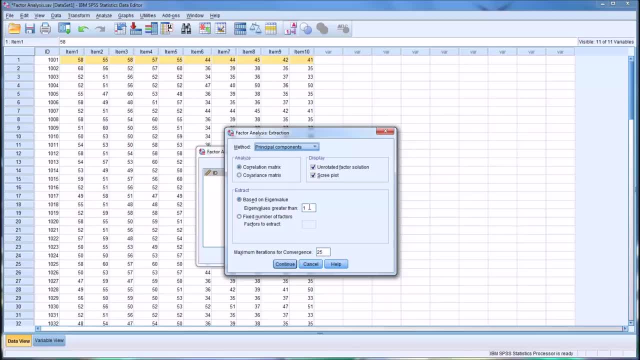 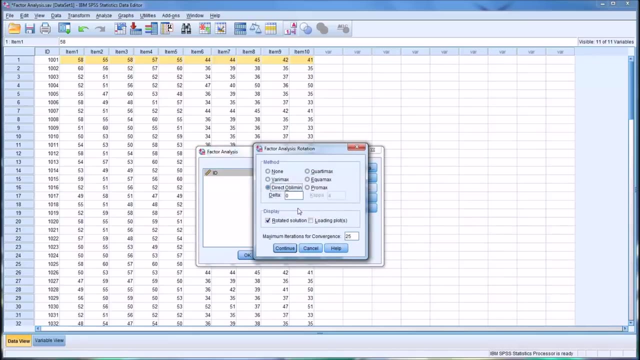 value of greater than one. so this is how it decides how many factors to extract, right so factors extracted if its eigenvalue exceeds one. now the rotation. there's a couple different types of rotations, actually several types of rotations, but there's two general categories right, and one is when 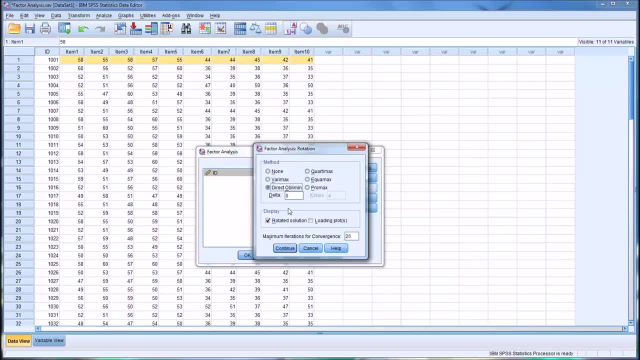 you believe that the constructs are unrelated to one another, so not correlated with one another, and one where you believe that they are correlated and there's a lot of different views on what type of rotation to use and of course it affects your results. but in the social sciences and counseling, for example, it's hard to. 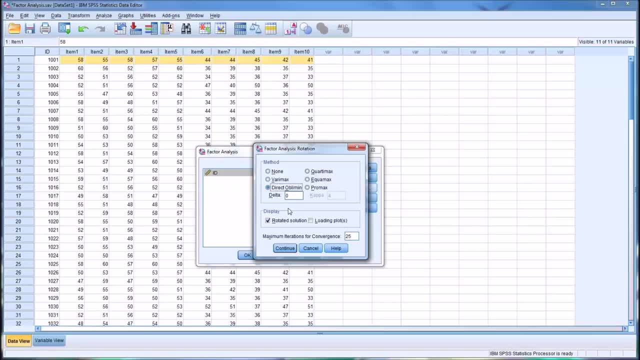 imagine a data set where you would have uncorrelated items. right, we know that in this particular instrument, we believe that the depression related items are going to be correlated to one another and we believe the anxiety, anxiety related items are going to be correlated one other, but also those two groups of items, rights, are going to be correlated to. 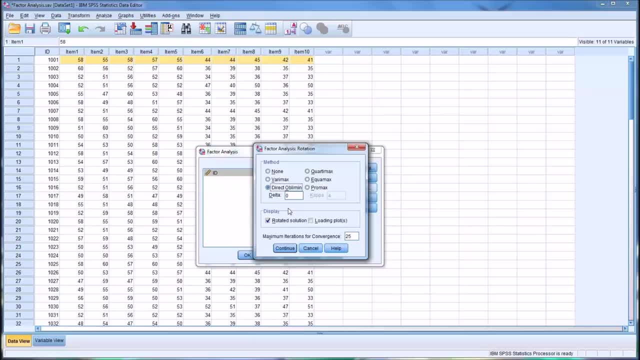 each other. so, for example, you know, item seven still might be related to item for, even though they load on different constructs. So in social sciences we tend to use- well, I tend to use- oblique rotations and I chose the direct. If you believe they're uncorrelated, there's a different set of options which we refer to as orthogonal right. 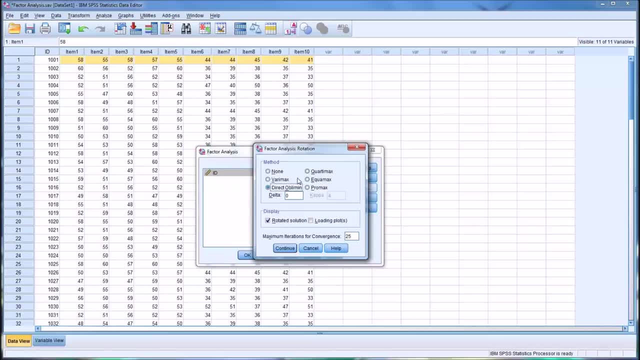 So that would be varimax, quatermax, equimax, And orthogonal means unrelated. so this is so it's easy to remember in that way: It's orthogonal if you believe that they're not correlated and it's oblique if you believe that they are correlated. 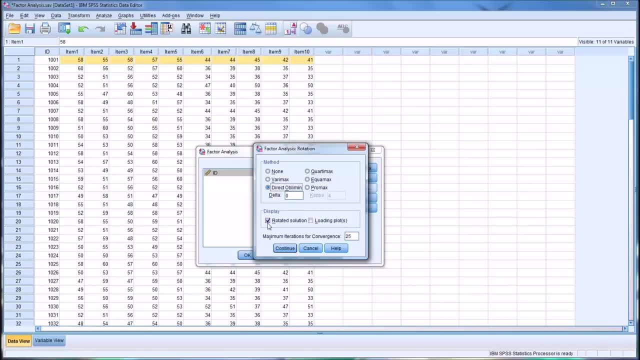 So I selected the direct and I want the rotated solution to be displayed. Scores: I did not endorse any of the options here, but you can save the scores. There's separate variables. And then for options, I left excluding cases list-wise, which of course, in this demonstration no cases will be excluded because all the data is populated. 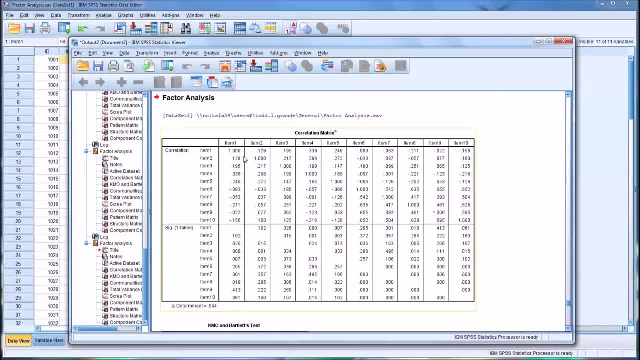 So then at this point you hit OK and you first see the correlation matrix. So, remembering our initial hypothesis about what we would find here, if you look at this matrix you can see that basically, item one is going to correlate perfectly with item one. 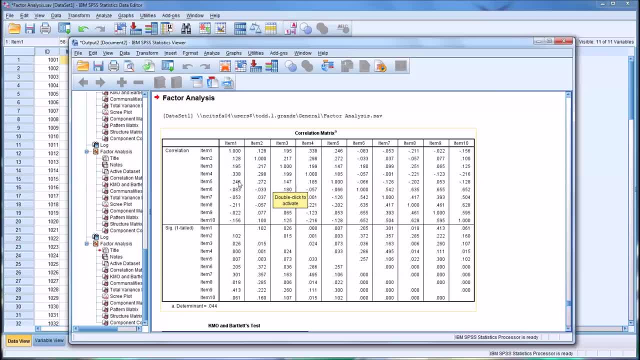 But we're looking for correlations between these different items. So item two: 0.128 with item one, Item four: 0.338,. so much stronger correlation with item one. And similarly, if you look at item six, you can see item six. 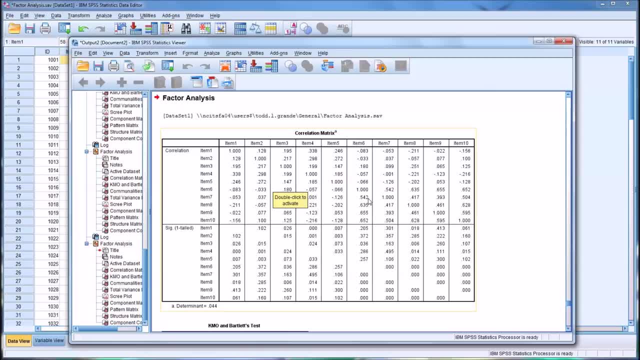 the correlation with item seven quite strong: 0.542.. And item eight and item six, 0.635.. But the other correlations are fairly weak, meaning the ones between depression and anxiety. So item three, correlating with item seven, for example, is fairly weak, but not in every instance. 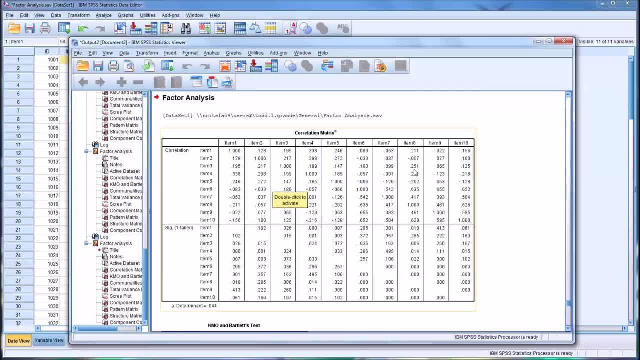 See item three. here correlates fairly strongly- Well, moderately- with item eight. So what we're really looking for here is a few things. We want to make sure that the items are correlated Like it gives us an idea of what's going on. 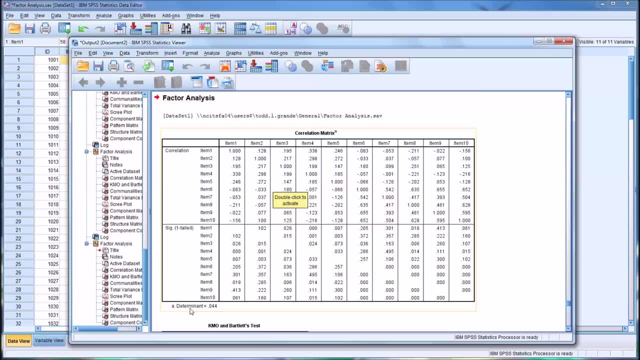 But we're really looking at the determinant right, And the determinant value here is 0.044.. This is one of the variables we're looking at. It has to be greater than 0.004.. It has to be greater than 0.0001, so we're fairly safe here with the determinant of 0.044.. 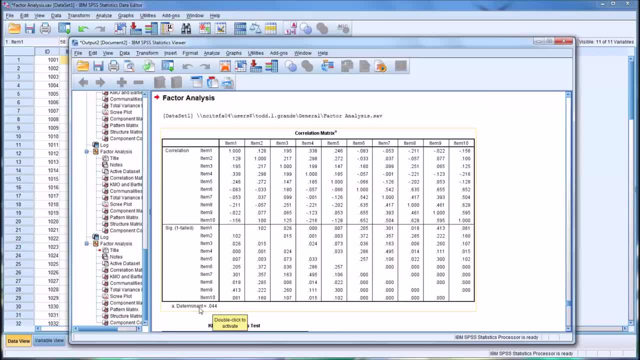 If it was below 0.00001,, then the items are too unrelated. the correlation is too low. Another area we want to look out for is correlations that are too high, what's called multicollinearity- Right When two items are really. 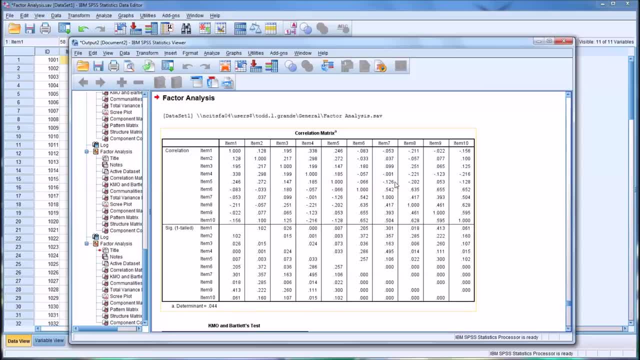 the shared variance is too high. they're explaining the same thing. that's not helpful either. And the cutoff for considering an item multicollinear in a factor analysis. one cutoff that's popular is 0.8, a correlation of 0.8.. 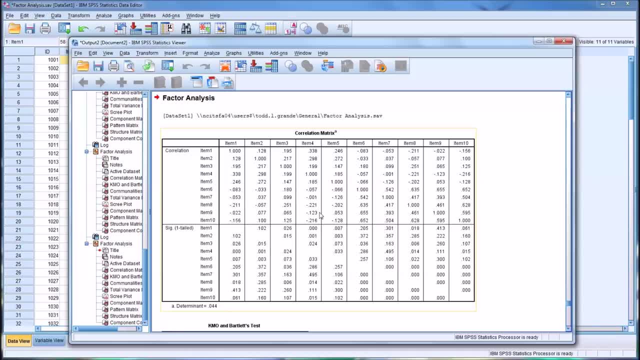 And you can see that none of the values here in our correlation matrix exceed 0.8.. If you have a perfect correlation outside of the, you know obvious. item 1: perfectly correlating item 1,. item 2: perfectly correlating item 2,. 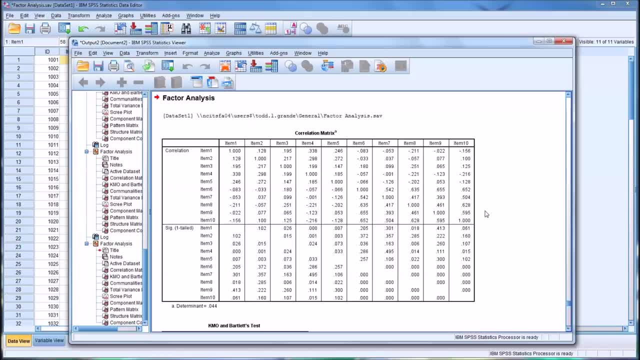 if you have a perfect correlation, that's called singularity And obviously in either one of those circumstances that presents a problem: either multicollinear or there's a singularity and you're going to want to remove that item from the analysis. 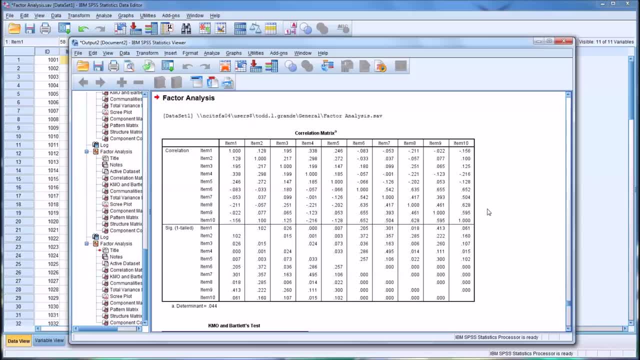 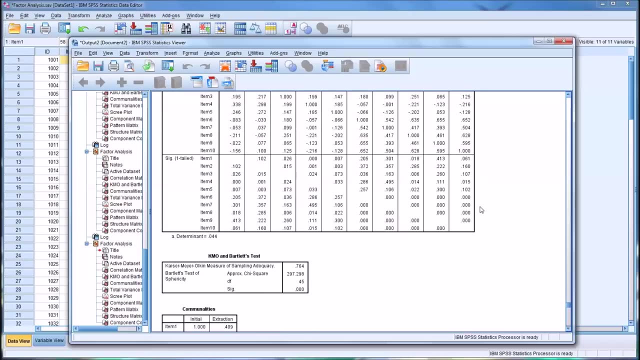 So a correlation of greater than 0.8,. you're going to want to remove and change around items to eliminate that item or one of the items in that mix. that's resulting in that high correlation. Looking at KMO and Bartlett's test, you want 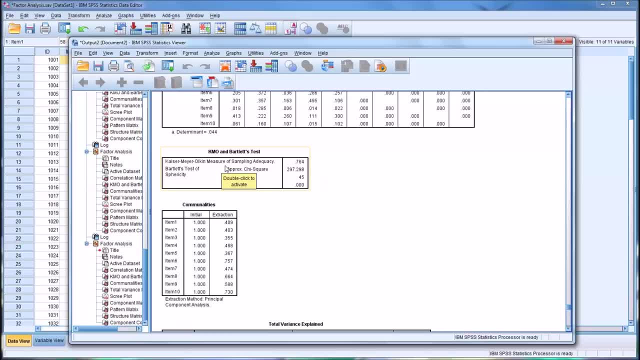 we have a value here for KMO of 0.764.. Anything above 0.5 is okay. Obviously, the greater the value here, the better. Similarly with Bartlett's test of sphericity: you want statistical significance and we certainly have it here. 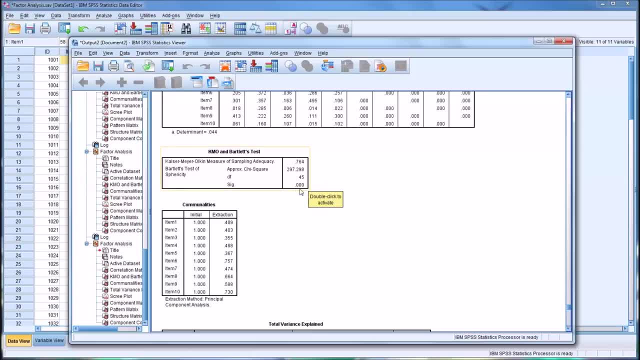 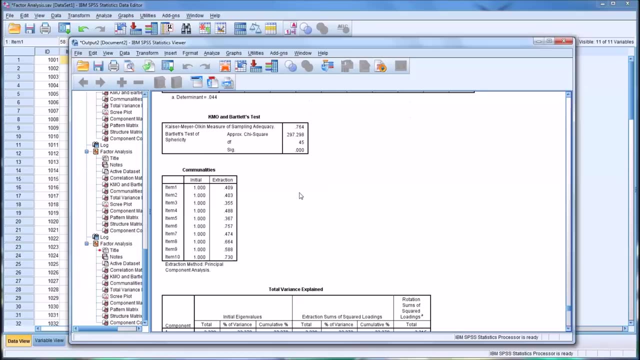 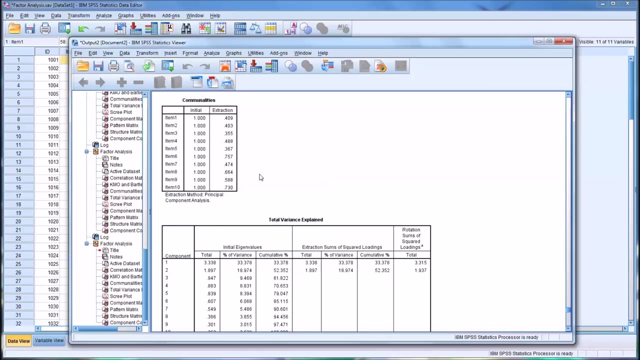 You can see it's 0.000, which usually for writing up APA-style papers. I record this as 0.001.. So a value less than 0.001 p-value. So you can see that the looking at the extraction here. let me move down. I'll come back up to the variance explained. 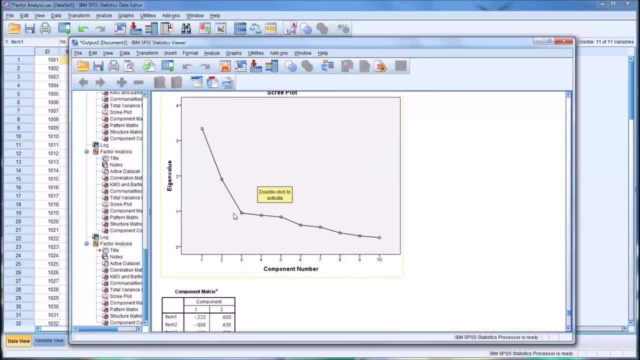 You can see that there's two components that were extracted based on the eigenvalue of greater than 1.. This is the eigenvalue of greater than 1.. This is the discrete plot. here You can see you have 1,, 2,, but this third potential factor didn't meet the cutoff. 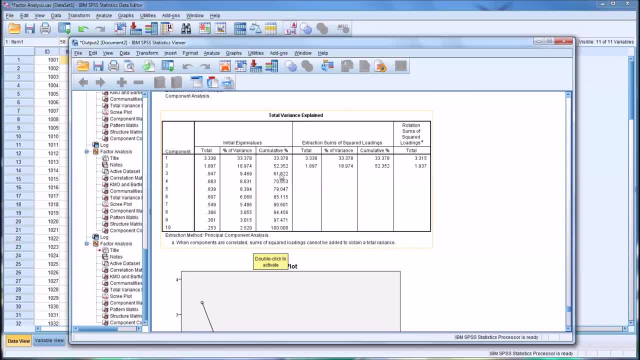 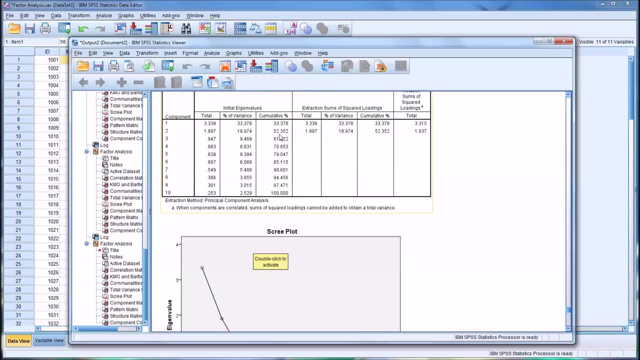 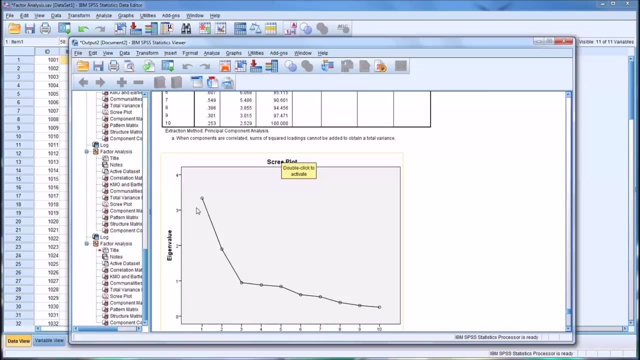 So these two components moving back up to total variance explained, explain 52% of the variance. So not ideal. Certainly a larger number here would be better, But still you can see from the discrete plot they are above the eigenvalue of 1.. 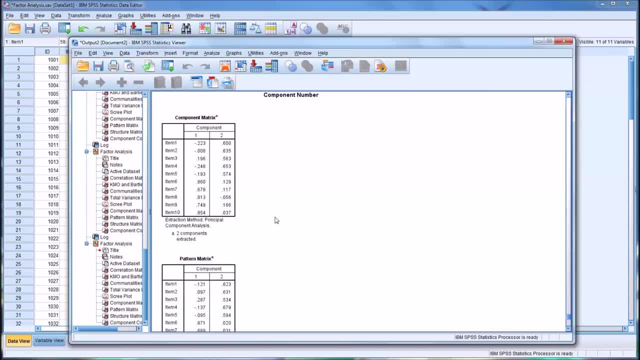 Now, since we used an oblique rotation, the direct, we're going to want to interpret the pattern matrix. It's not a whole lot different than the component matrix or the structure matrix, But this is the one we're going to want to look at with this particular rotation. 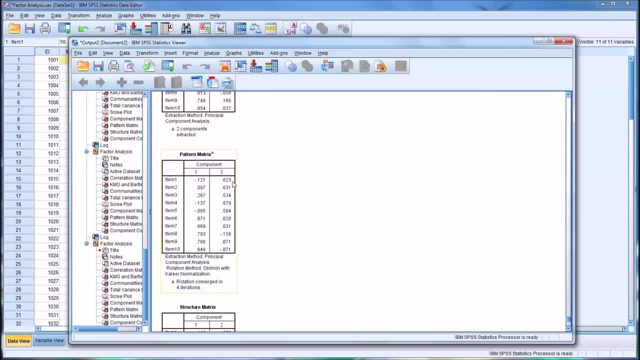 And you can see- let's start with component 2,. you can see these values load together fairly tightly. These seem to represent one construct as you look here. There's not a lot of variance here. Similarly, we believe that items 6 and 10,. 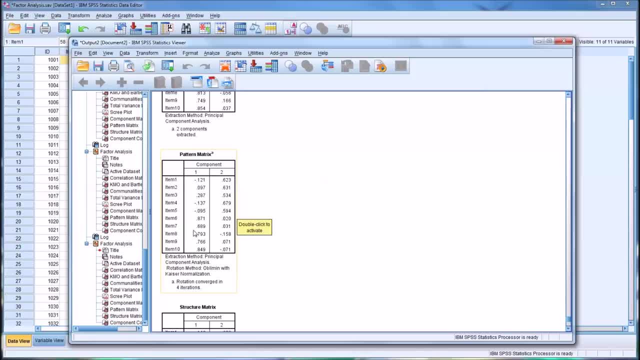 represent a construct. In the case I have here, it was supposed to be anxiety, right, And you can see again. these load together fairly tightly. So if you look at this pattern matrix, there does seem to be two distinct factors.